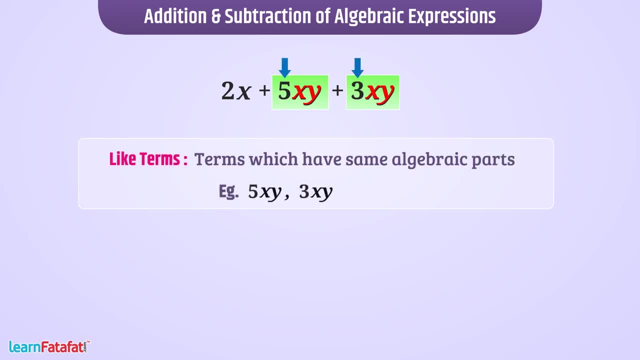 irrespective of coefficient, are like terms. If we compare 2x and 5xy, then here algebraic parts are not same. Such terms are called unlike terms. Since algebraic parts are the same in these two terms, we can take the algebraic factors common as 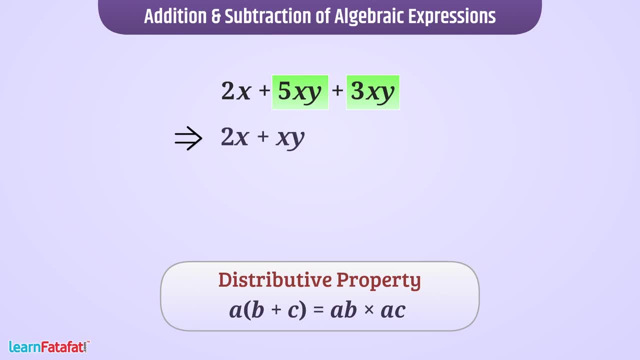 per the distributive property. 2x plus xy multiplied by 5 plus 3 is equal to 2x plus xy into 8, which gives us the expression 2x plus 8xy. We can see that 8xy is also a like. 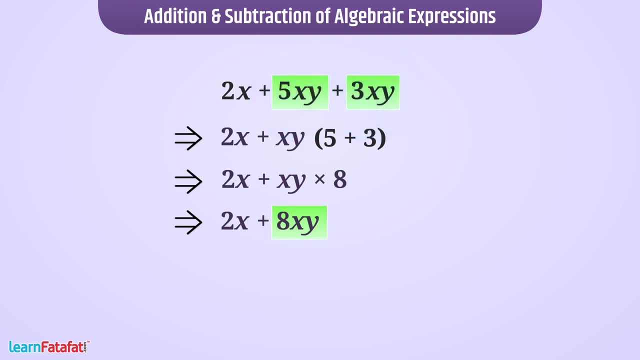 term as that of 5xy and 3xy. Thus the sum of two or more like terms is a like term, with a numerical coefficient equal to the sum of 5xy and 3xy. Now if we look at 2x and 8xy, we see that they don't have the same algebraic part, and 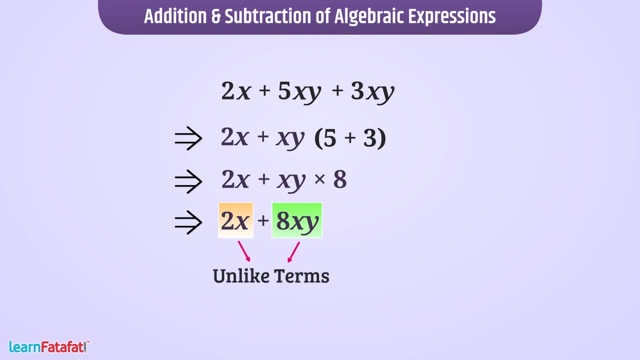 hence these are unlike terms. Can we simplify the expression further? No, because even if we take 2x common, still 1 and 4y cannot be solved. Thus we can say that unlike terms, unlike terms cannot be added. In the same way we can solve the expression 2x plus 5xy. 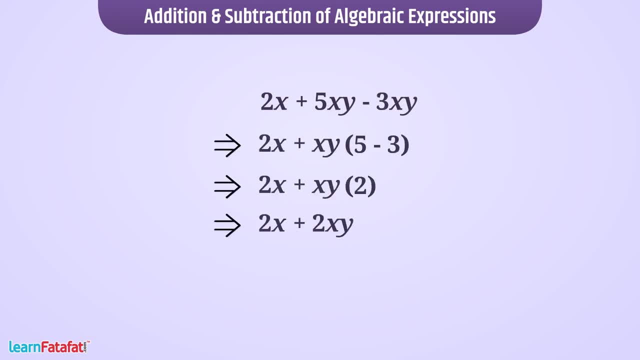 minus 3xy, as shown, From which we can notice that the difference between two like terms is also a like term with numerical coefficient equal to the difference between the numerical coefficients of two like terms. We cannot carry out subtraction on unlike terms. Let's 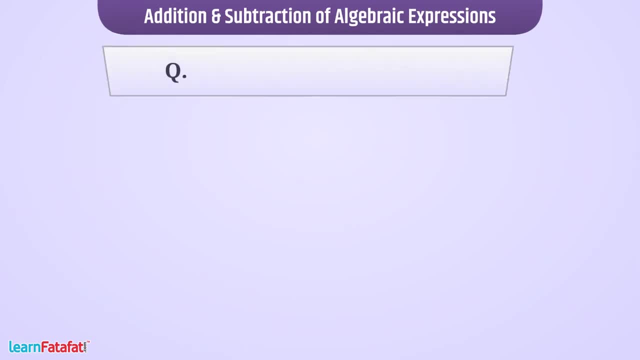 solve some examples. Add 3x minus 15 and 22x plus x minus 14.. We can write it as 3x minus 15 plus 22x plus x minus 14. That is 3x minus 15 plus 22x plus x minus 14.. Then we rearrange the terms. 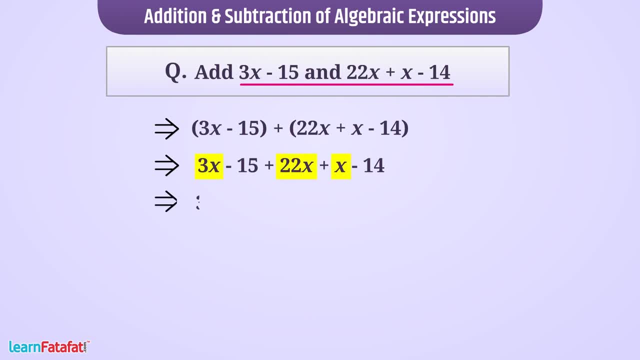 such that, like terms come closer, 3x plus 22x plus x minus 15 minus 14.. We can take algebraic parts common: x multiplied by 3 plus 22 plus 1 minus 15 plus 14.. x multiplied by 26 minus 29. That is 26x minus 29.. 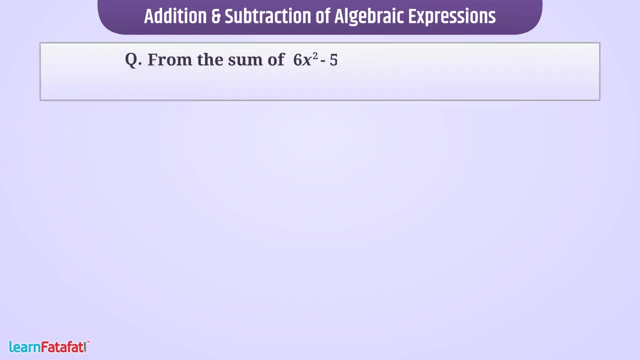 Next example From the sum of 6x square minus 56xy plus 32x minus 29.. We can take the algebraic parts common 3x plus 32x minus 12 and 4xy plus 15, subtract 5x square plus 3xy minus 34.. We can solve: 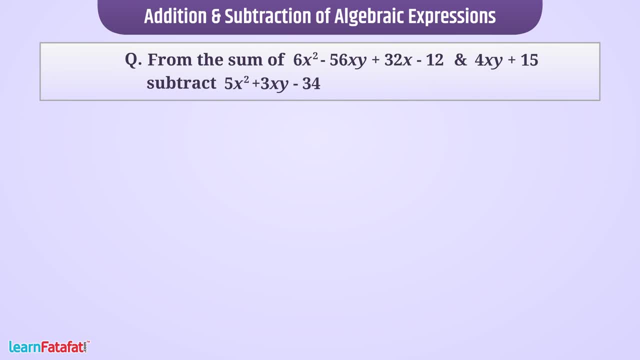 it as we have done in earlier example. But through this example we will learn a different method. First we will add these two expressions to find their sum. For that we will write the first expression as it is and then we will write the second expression below it. 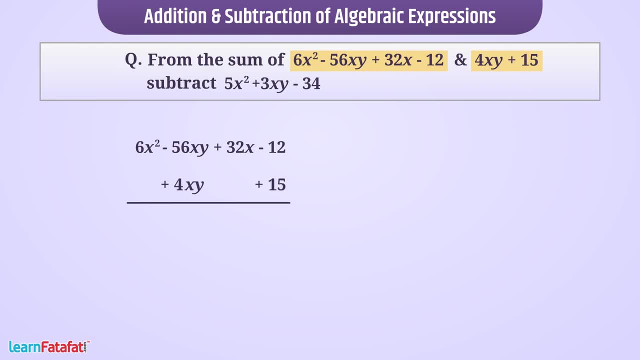 below it, such that the term appears exactly below like terms. We will add two expressions, as shown. This is the sum of these two expressions. From this sum we have to subtract this expression. We will follow the same method. First we will write the expression from which the other expression is to be subtracted. 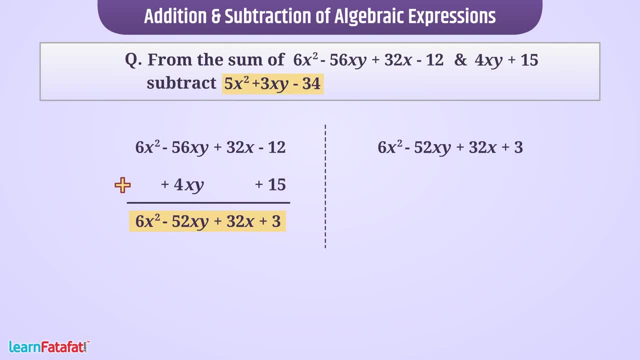 Then we will write the other expression below it, such that the like terms will be exactly below the like terms. Note that subtracting a term is same as adding its inverse. So here, subtracting 5x square is same as adding minus 5x square. 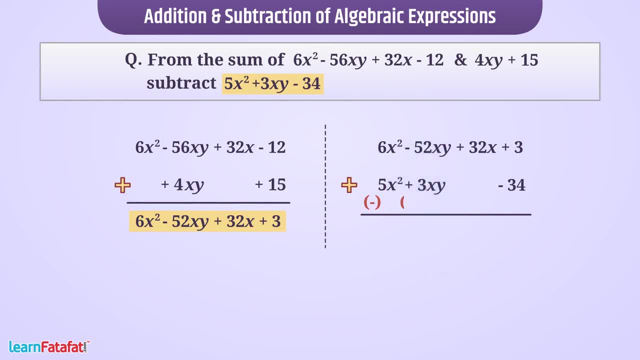 Similarly, subtracting 3xy is same as adding minus 3xy and subtracting minus 34 is same as adding 34.. So, addition of 6x square and minus 5x square is x square. Similarly, addition of minus 52xy and minus 3xy is minus 55xy. 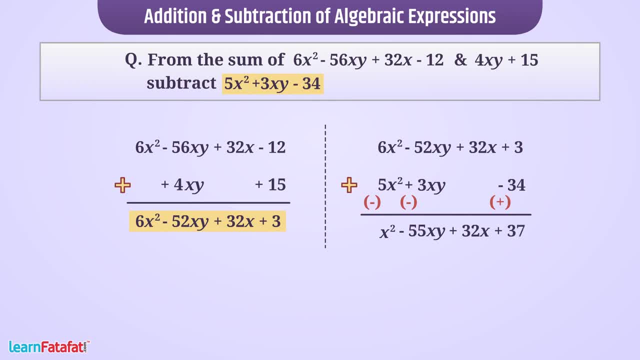 Likewise we will get the result as x square minus 55xy plus 32x plus 37.. I hope now you can add and subtract algebraic expressions easily. Thanks for watching this video.